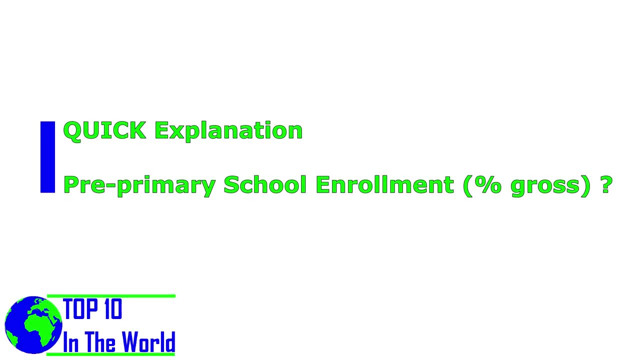 Pre-primary education refers to programs at the initial stage of organized instruction designed primarily to introduce very young children to a school-type environment and to provide a bridge between home and school. Thanks for watching, guys, remember to subscribe and like to keep the channel alive.